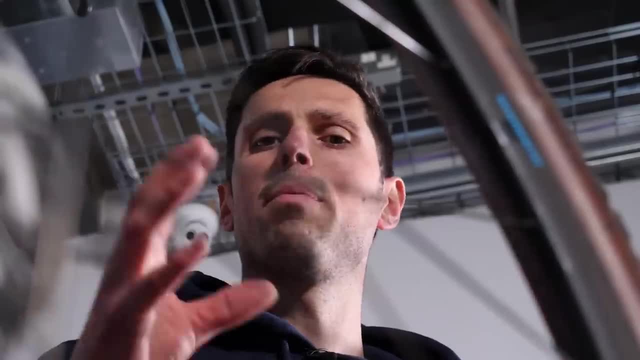 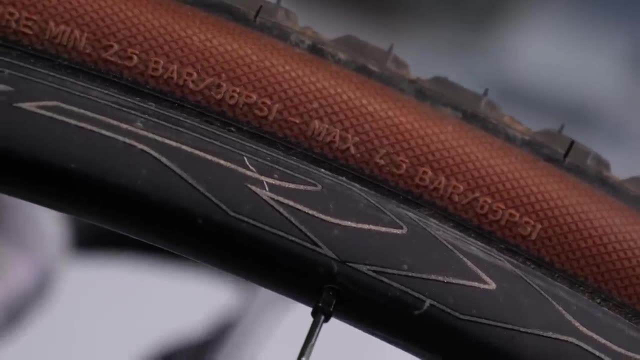 you're probably going to want to look to check this once a week. That should be a pretty good starting point for most setups. In terms of the pressure now, this is going to vary quite a bit depending on the setup that you have on your bike, the width of the tire and the weight of the rider. As a general starting point, a 25-millimeter road tire. with an average weight rider running it in a tube, you should probably look in the region of around 100 PSI. A lighter rider, you could reduce that pressure down slightly. A heavier rider: increase it up a little bit more. Now on an even wider tire, such as this gravel bike I've got here. you could probably look to be in the realms around 30 to 40 PSI, but the best thing to do is to refer to the pressure chart supplied by the manufacturer of your tires. I'll put up on the. 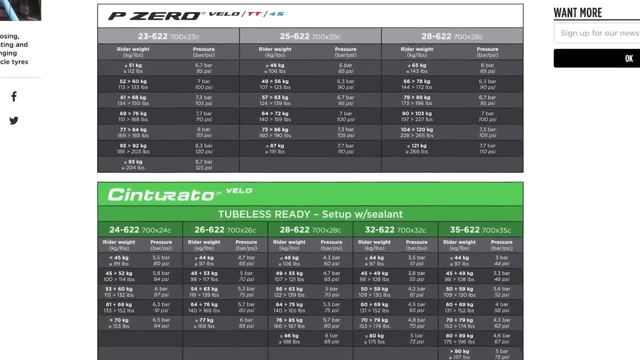 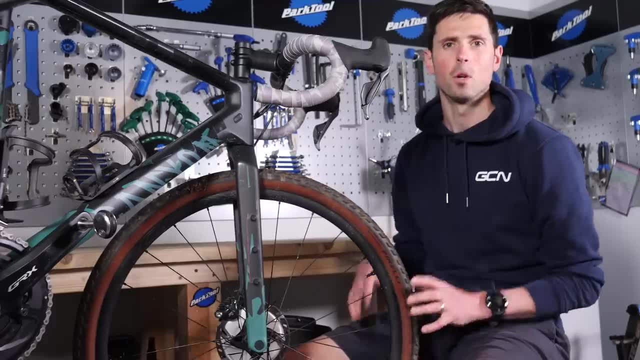 screen the pressure chart supplied by the manufacturer of your tires. I'll put up on the screen a chart which gives an indicator for Pirelli road tires. You can see as the width of the tire and the weight of the rider changes, so does the recommended tire pressure, Almost all. 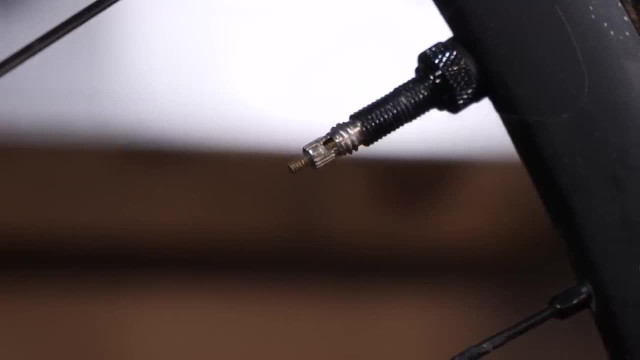 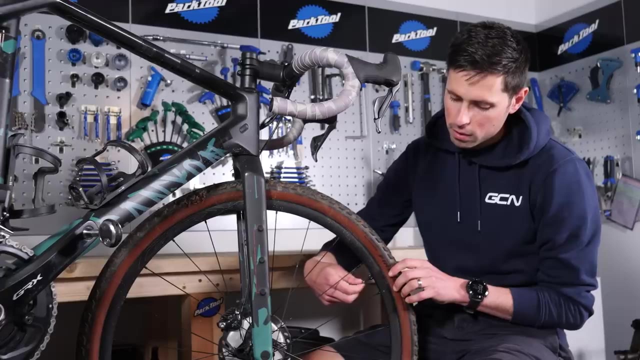 bikes will have a valve which looks like this and it's referred to as a Presta valve, To pump the tires up. that uses this valve. you need to undo this small little end cap on the valve until that's nice and free. Take your pump which has the suitable Presta valve fitting. 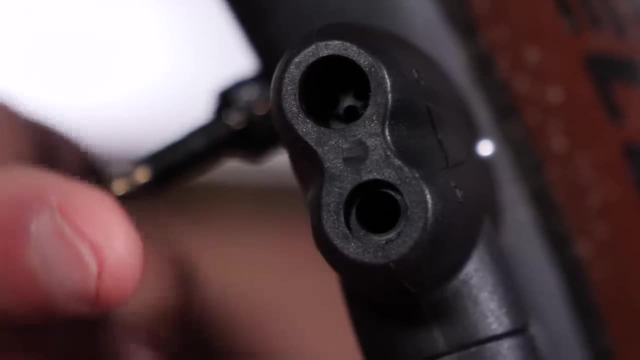 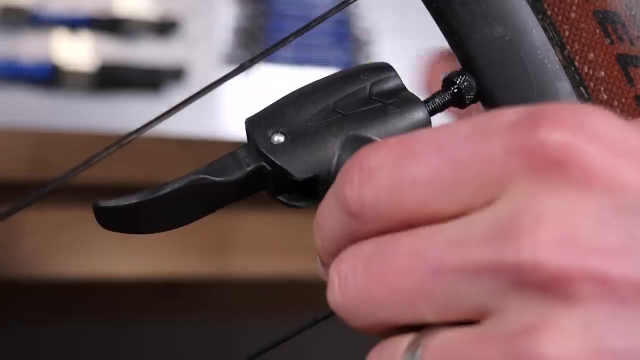 If you've got two options on there, it's the smaller of the two- Place it all the way over the valve, push it firmly into place and then pull the lever all the way back. At that point you can pump away to your heart's content using your pump to set it to the correct. 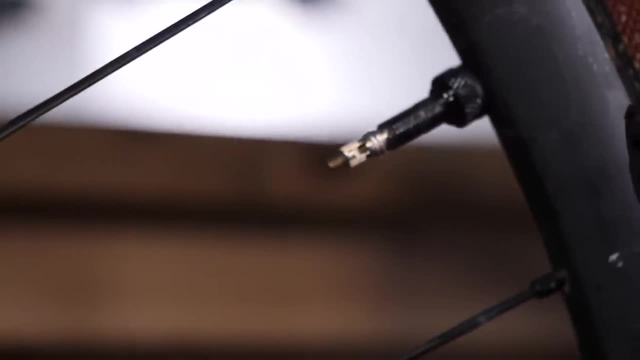 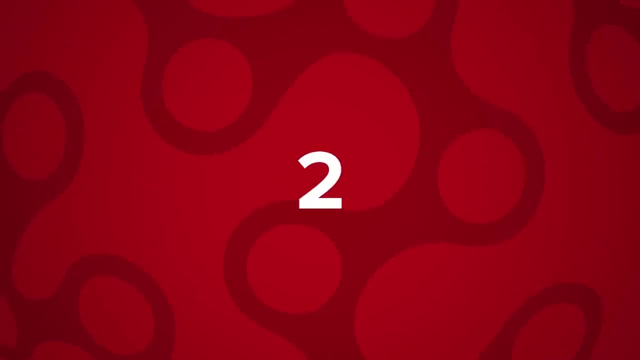 pressure. Oh, and, when you take the pump off like this, don't forget to do the valve back up. No need to do it super tight. Finger tight is perfect. Thankfully, cleaning your bike is a pretty simple process as well. You're only actually going to. 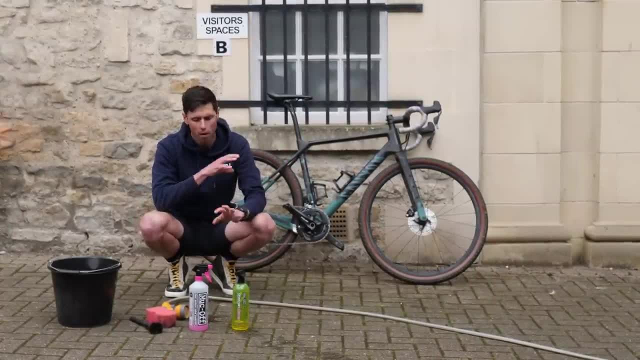 need a few minutes to clean your bike. You're only actually going to need a few minutes to clean your bike, A few components to do the basic job. Although there are a whole host and plethora of fancy pants, cleaning products out there, you only need some of the essentials. 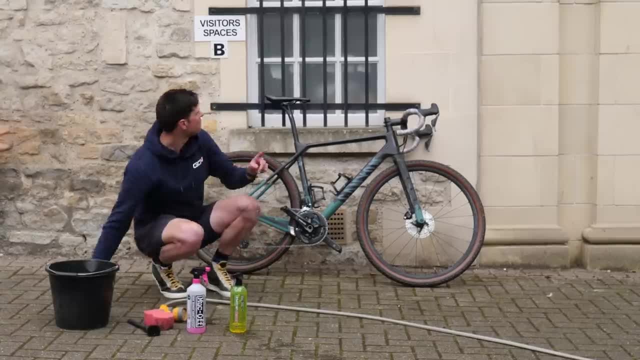 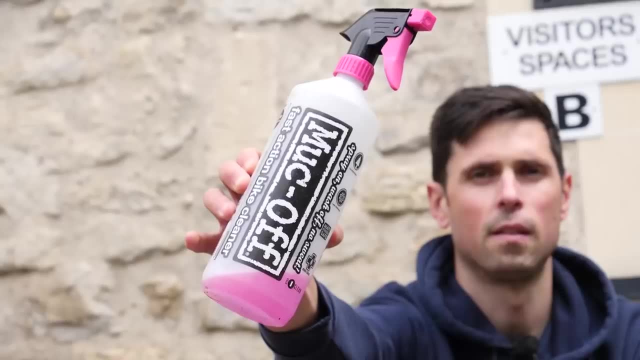 to get the basic job done. Something that you definitely don't need is to book out Visitor Space B. I've just done that for today. Now, the things I've got in front of me are the general purpose bike cleaner. I've got a degreaser. best to use a bike-specific one. 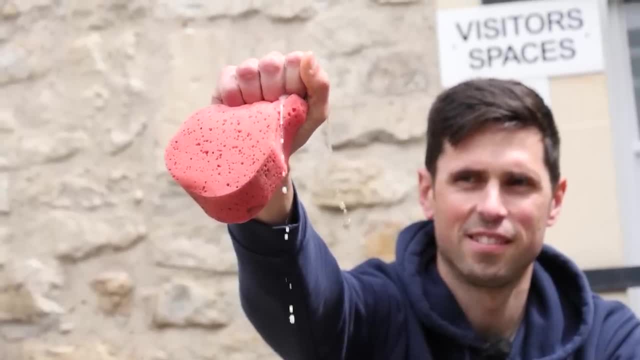 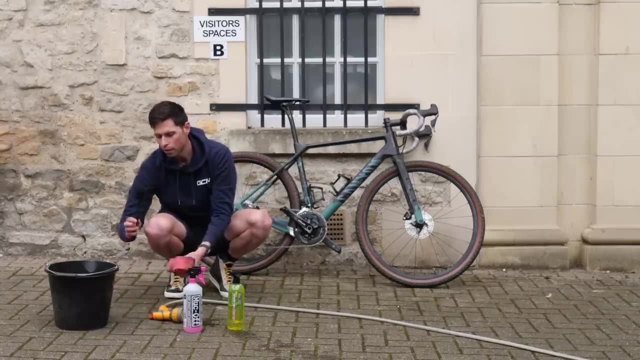 and then I've got a clean sponge and a brush. Now you need to have one or the other. You can either have two brushes or two sponges or, as I've done, gone for a mix. One of them you're going to use to clean the frame and many of the cleaner parts. 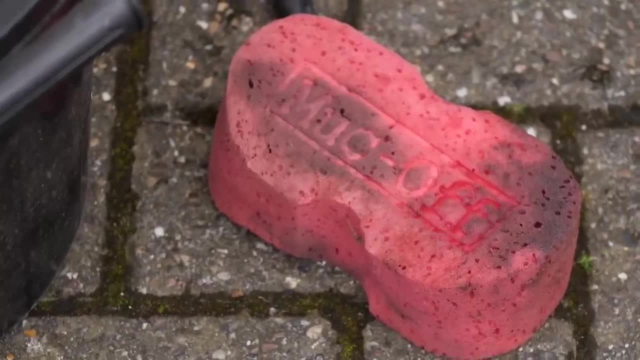 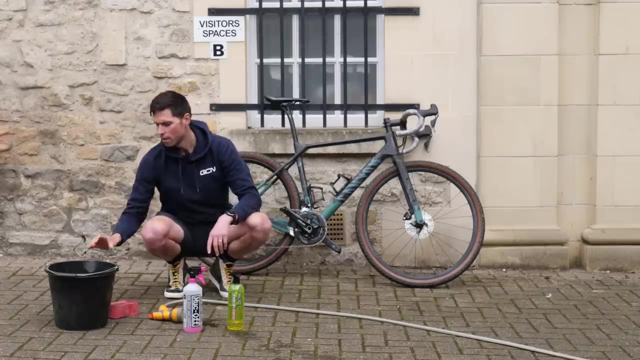 of the bike. You're going to keep that nice and free from grease. Then I'm going to use the brush to clean all the chain, the cassette, the chain rings, all the bits that are pretty grimy and horrible. Then I've also got my bucket. If you've got access to a hosepipe, happy days. 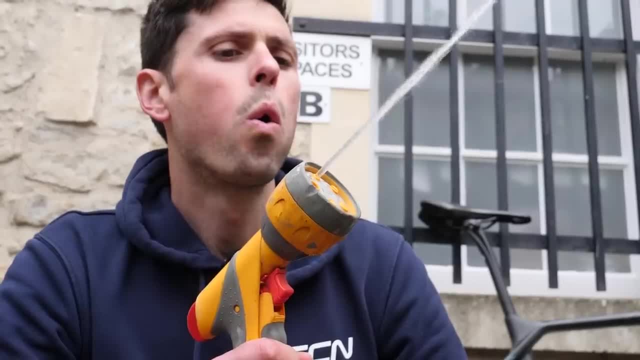 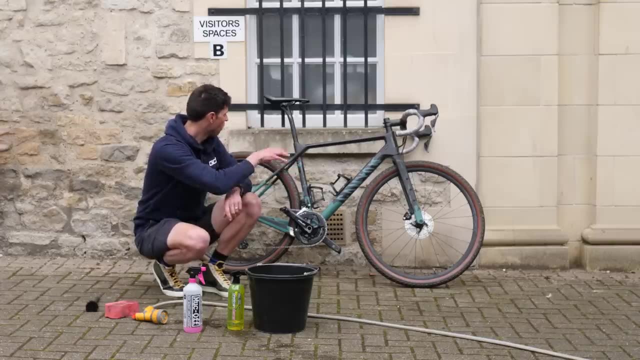 You can use that for your clean water supply, or you can just fill your bucket up a couple of times. First thing we're going to do is to use our hosepipe to simply wash off all of the loose dirt and get all of the easy bits off. we can do first, Let's do it. 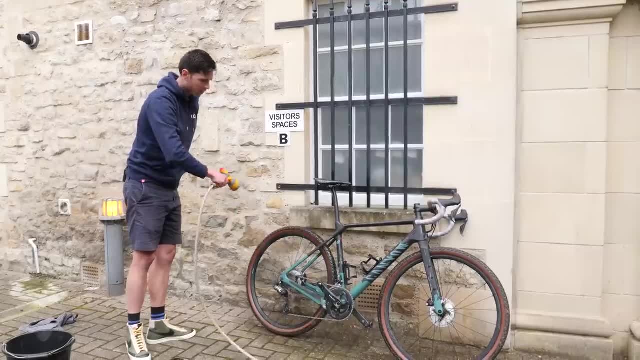 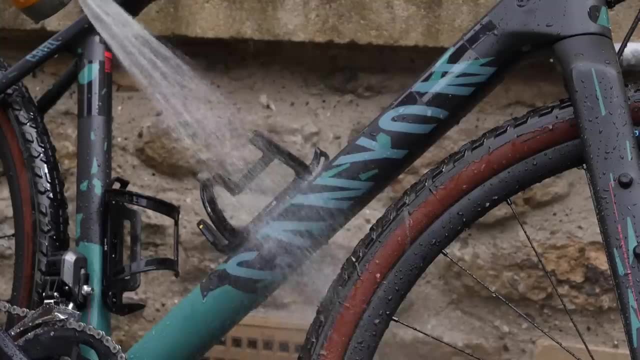 Using a hosepipe, blast off and soak all of the bike. If you clean the gravel bike like this, it's a good idea to let the moisture soak into some of the mud to loosen it off. Then you can use a little bit of the pressure to blast off the loose sections. 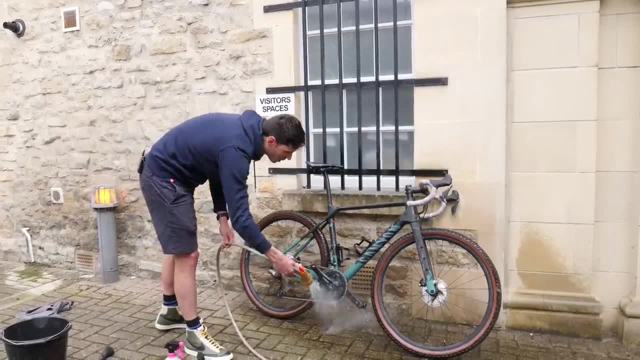 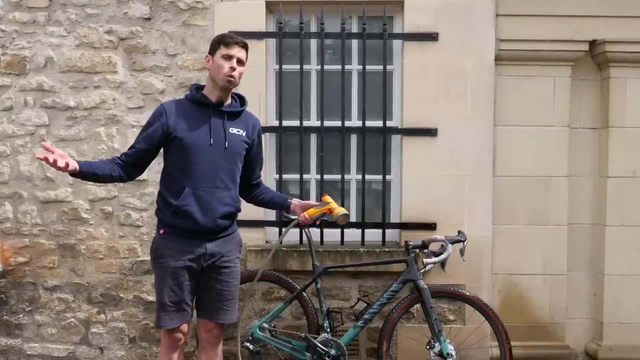 Don't forget all the little bits underneath the saddle and underneath the bottom bracket. Job done. If you haven't got a hosepipe, you could just use a watering can or your bucket and then pour all the water over to get all the loose bits of dirt off. To apply your bike cleaner or detergent to the bike. 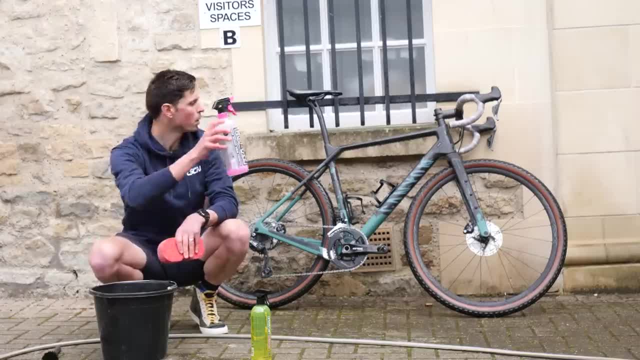 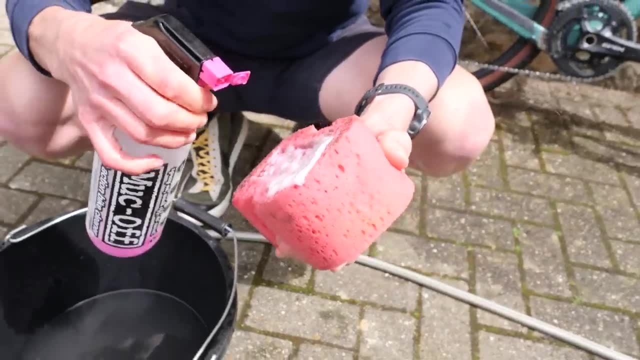 you've got a few options. Option one: spray it directly from the bottle all over the bike. Option two: spray it directly onto your sponge or brush. Option three: pour the relevant amount of liquid into the bucket, although that's going to use far more up. What I'm going to do to save. 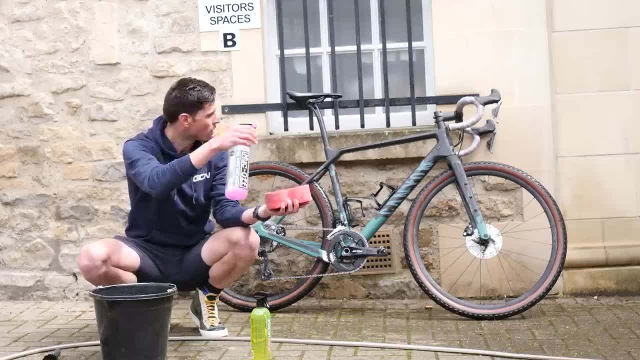 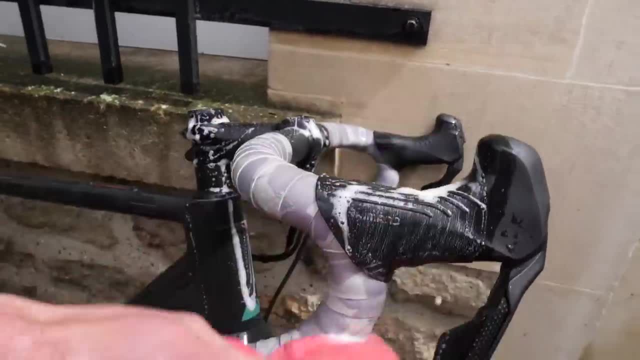 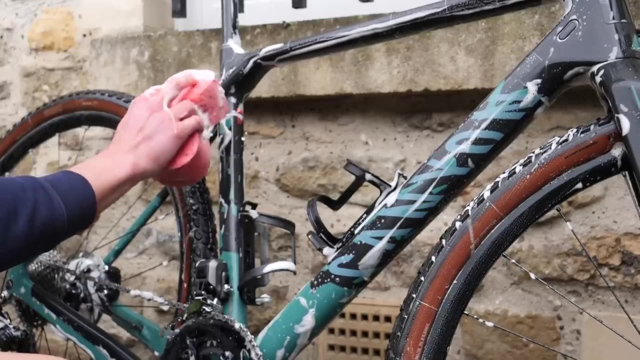 you using loads. I'm going to spray it directly onto my sponge and then work the sponge all the way around the bike. Let's do it. It's a similar situation for your degreaser. You can spray it directly onto the bike or 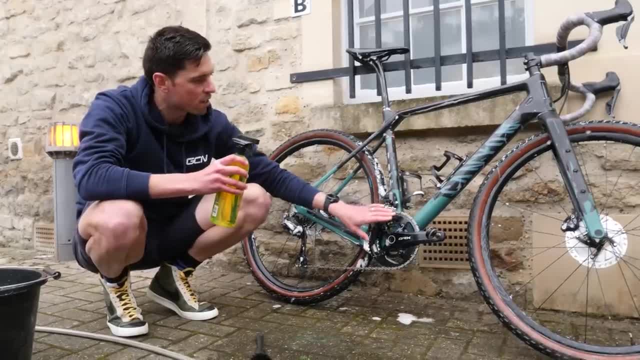 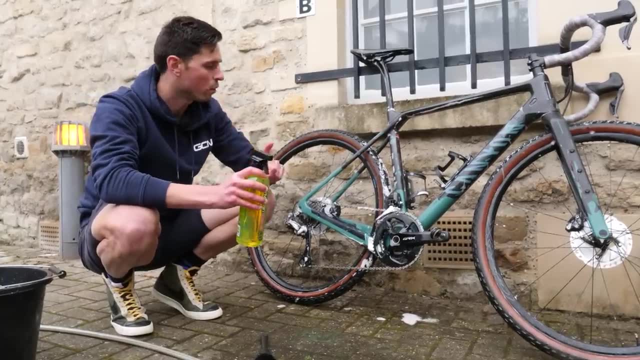 spray it onto your brush. What you need to do is ensure that you get degreaser over the chainrings, the cassette and all the way around the chainring Speaker 1 chain, including the pulley wheels, but be mindful not to spray it directly into your. 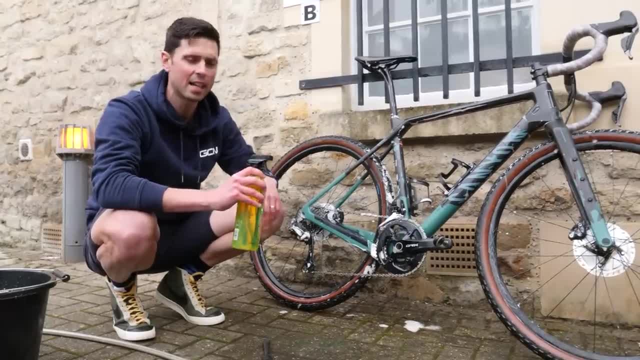 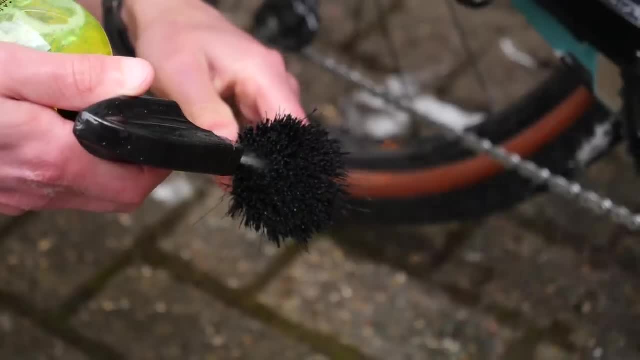 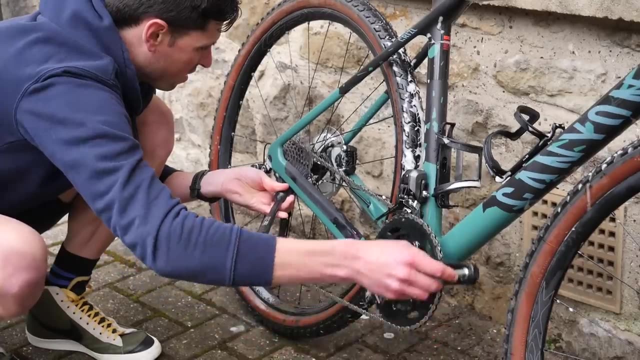 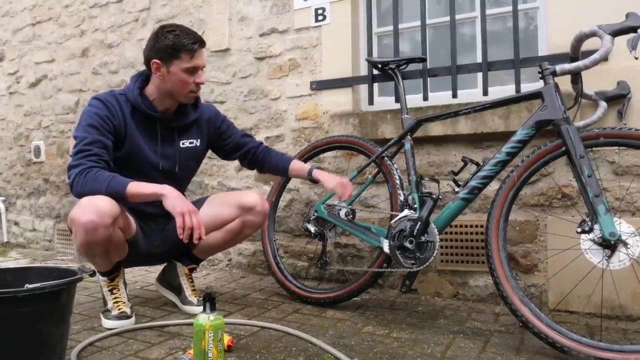 bearings, because I lost count how many times people have commented: God, look at Alex spraying degreaser into all his bearings. Just take a bit of caution. That's the frame, the wheels, all of the bike clean. We've gone to town on the drivetrain. let the degreaser work its magic and 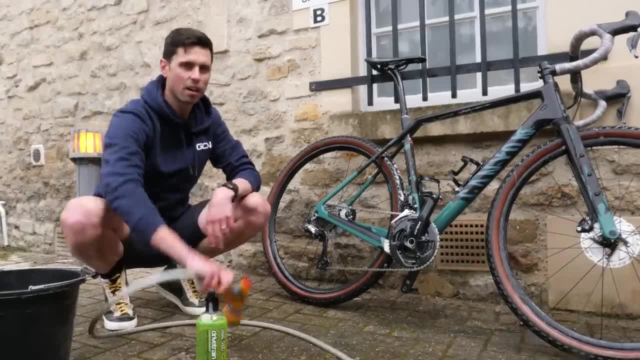 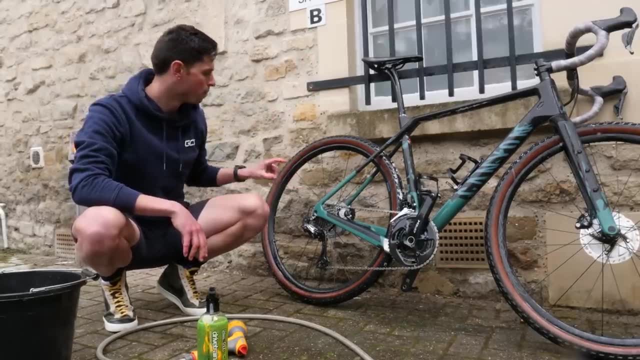 agitated that all the way in. The next stage here is to take our hose pipe or our bucket of fresh water, rinse all of the soap suds in the degreaser off of the bike. Now, as we're doing the degreaser, 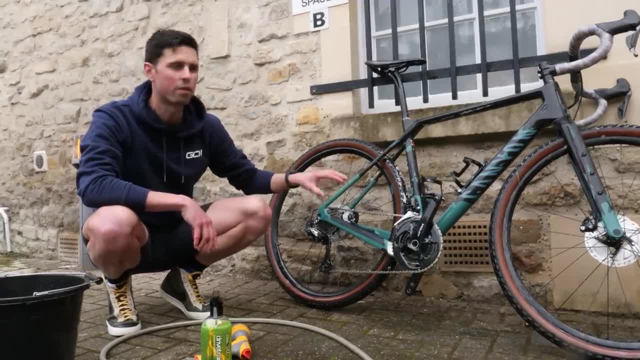 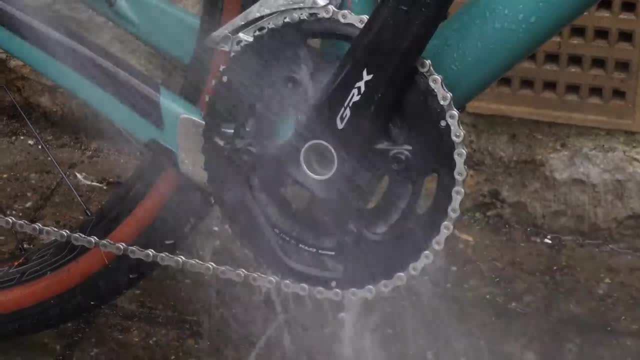 and getting out of the chain. we can backpedal as well to help wash all of that degreaser out. Then after that, flip the bike around, repeat the process. Let's do it Speaker 1 Pedal as well, like this: Speaker: 2 Speaker, 3 Speaker, 4 Speaker, 5 Speaker, 6 Speaker, 7 Speaker, 8 Speaker, 12 Speaker, 13 Speaker, 14 Speaker, 15 Speaker, 16 Speaker, 18 Speaker, 20 Speaker, 21 Speaker, 22 Speaker 23. 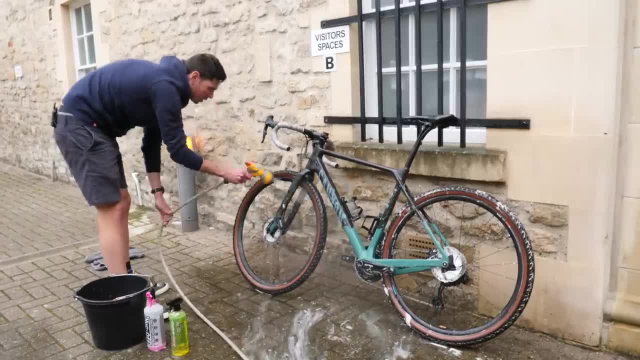 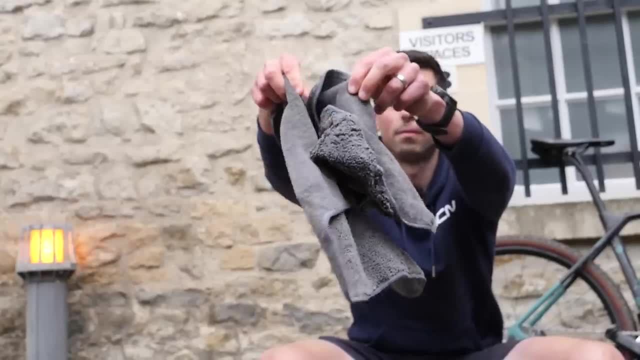 Speaker 24. Speaker 27. Final step of cleaning the bike. the bike is drying the bike. For that I've got two cloths, One which I'm going to use for the entire frame, the wheels and generally all the components that are fairly clean. 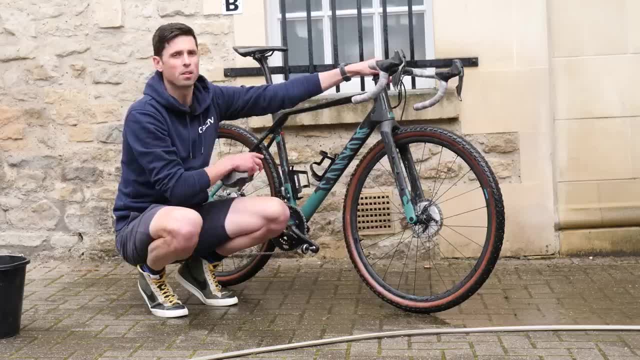 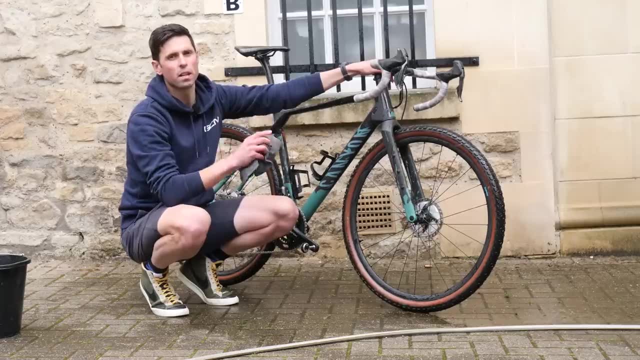 Then the other cloth I'm going to use to wipe down all the drivetrain components, so the chain, the cassette and the chain rings, so that I'm not going to spread any remaining grease or any other bits of dirt over the rest of my bike. Then I can keep those cloths. 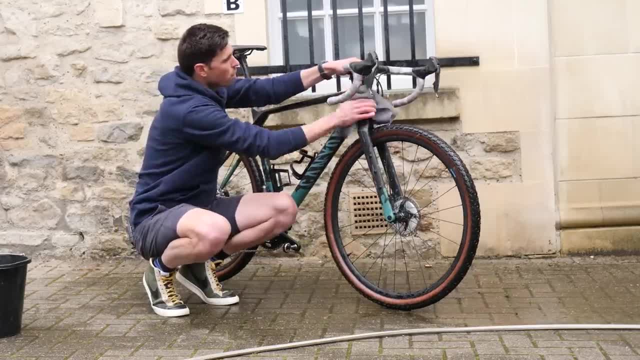 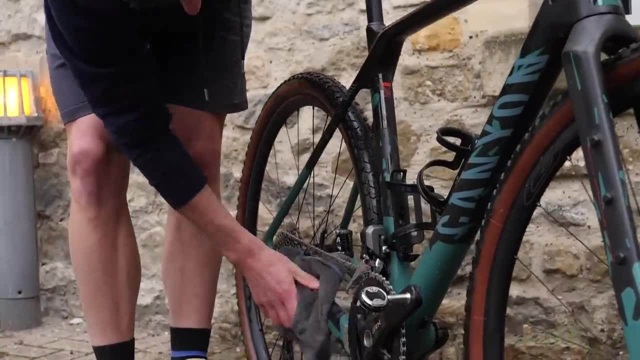 that order ready for when I next do the job. Let's get to it. Dry all the watery bits off, do our best to have a nice, clean bike and you also, at the same time, going to be able to examine how good- or maybe a bad- a job you've done at cleaning your bike for the first time. 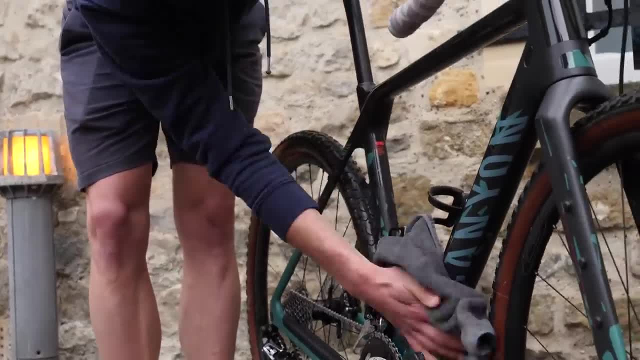 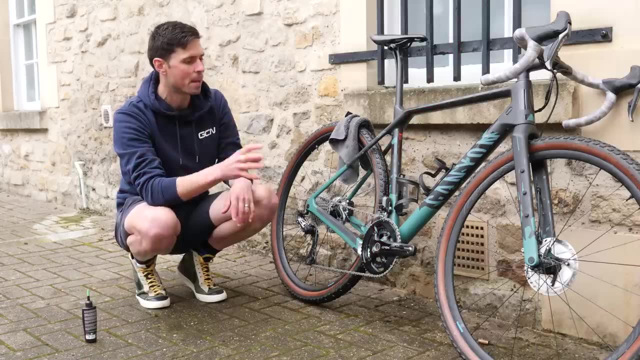 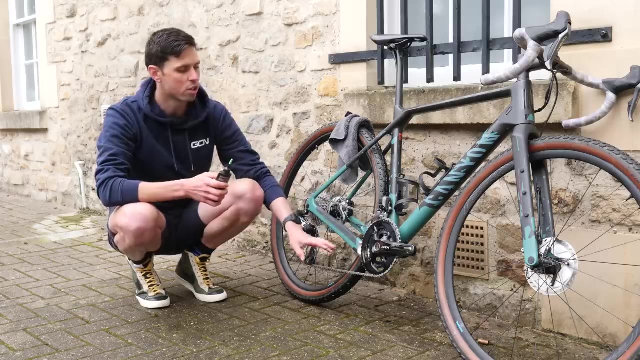 Don't worry about it. You'll only get better. Once you've cleaned the bike and dried it off thoroughly, the next step for the basic maintenance is just to lubricate the chain. You just simply need to take your favorite bike chain lube and apply it onto your chain. 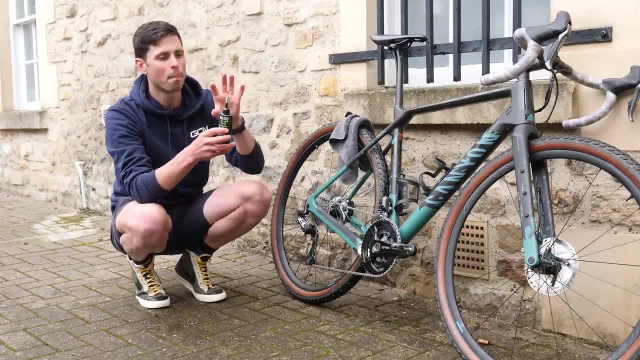 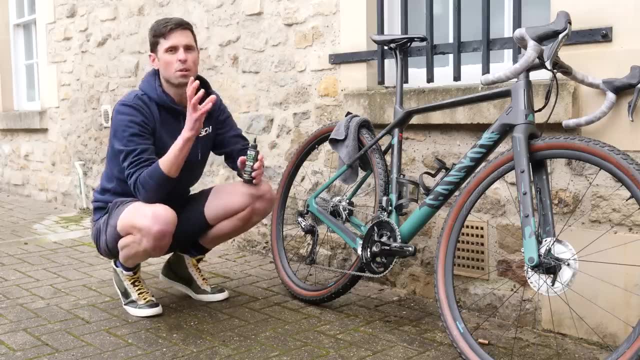 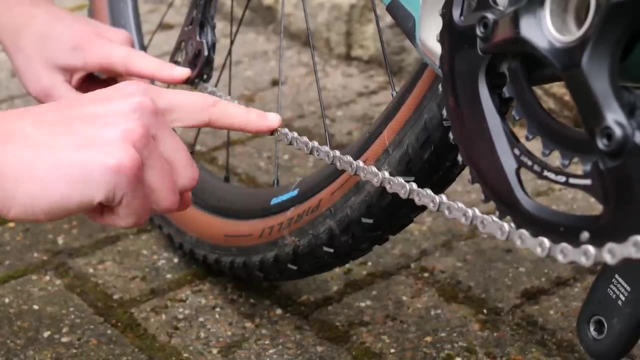 that you've just thoroughly dried. What we're trying to achieve is to get about one drop of chain lube on the inside edge of the chain for every single roller. Now, the easiest way to apply the chain lube is to simply backpedal the bike and apply the chain lube between the lower pulley wheel. 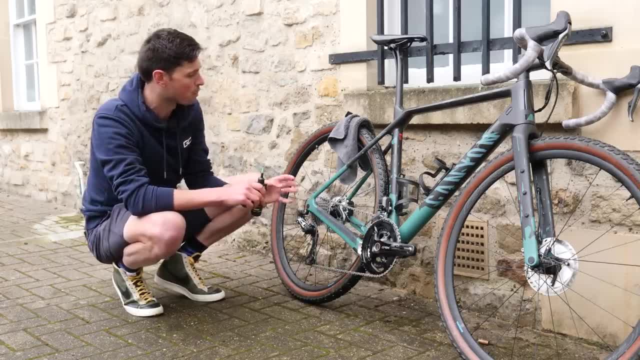 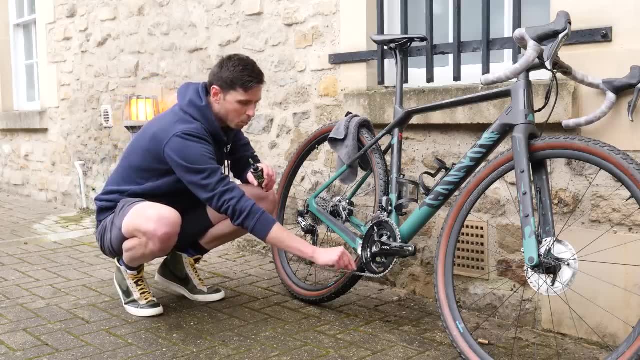 and the chain ring. This is because this is the surface that is in contact with most of the components most of the time. Now, if you've got three minutes of your life which you're willing to give away, you could individually apply one drop to every single roller. but